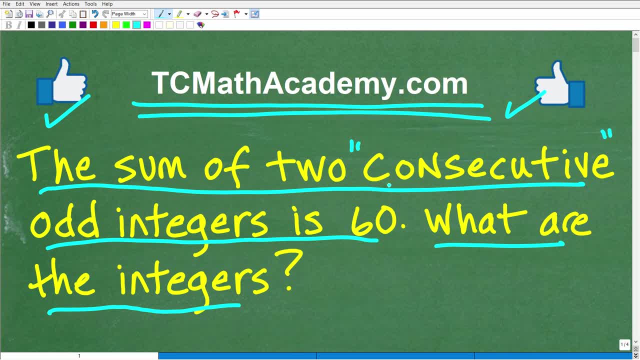 of students may not quite understand this word consecutive. They're like: well, what does that mean? And they may have forgotten what an integer is. No big deal. I'll explain this here in a second, But let's go ahead and take a look at the answer Again. we're looking for two integers. 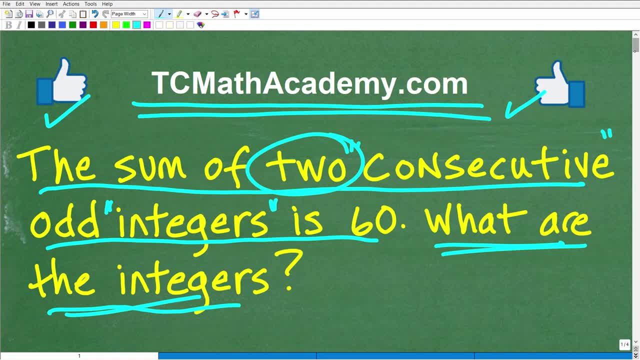 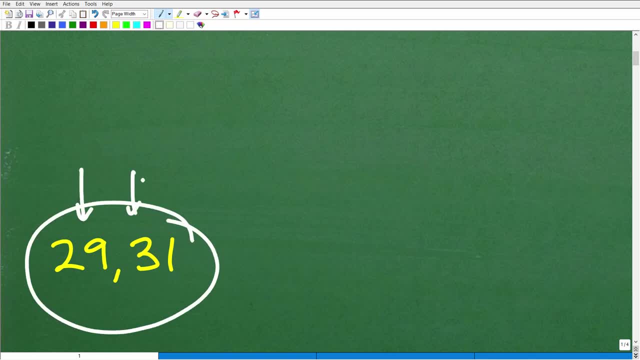 right: Two consecutive odd integers that add up to 60. So what is the answer? Well, the answer is 29 and 31.. These are your two consecutive odd integers. Okay, so how'd you do? Well, hopefully you got this right, If that's. 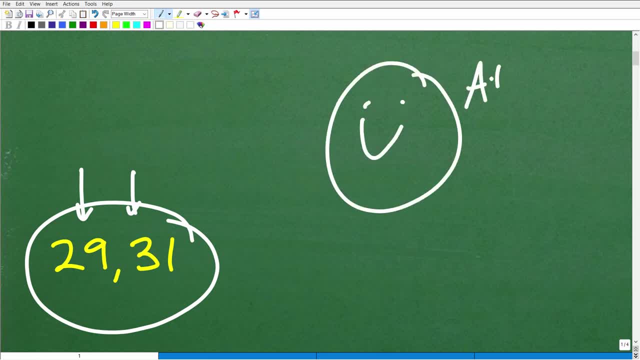 the case, let's go ahead and celebrate by giving you a nice little happy face, an A plus a 100% and multiple stars. You could tell your friends and family that today you solved an interesting algebra word problem. They'll be very, very happy and pleased to hear that information indeed. 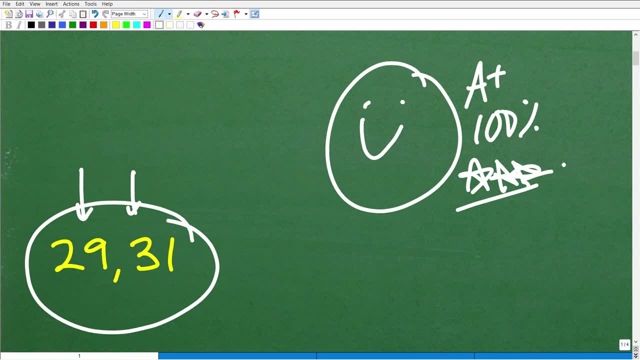 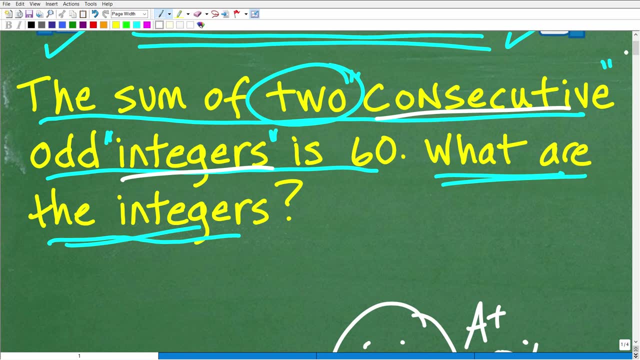 Okay now, if you are like: well, I'm confused because I don't know what this, you know what words mean, or you know, you're not quite sure what consecutive and integers means, well, obviously, you're going to have to have a really solid understanding of these terms. 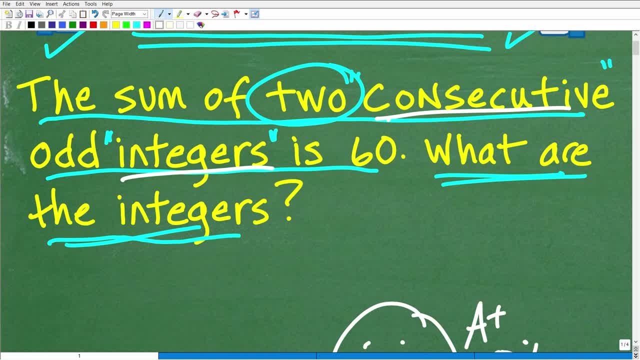 in order to solve this problem. Now, before we get into the actual problem, let me go ahead and just kind of stress to you that, you know, knowing having a strong math vocabulary, okay, is very important, Like you know. an integer, What is an integer? What is a rational number? You know. 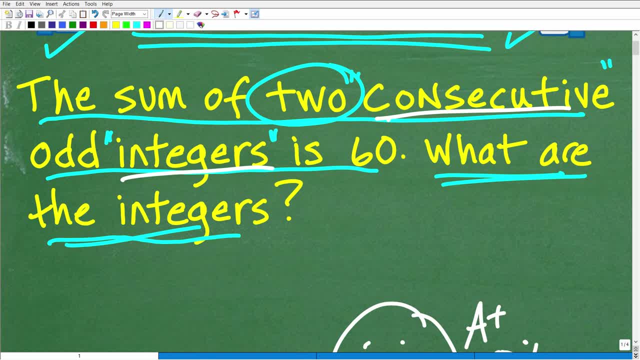 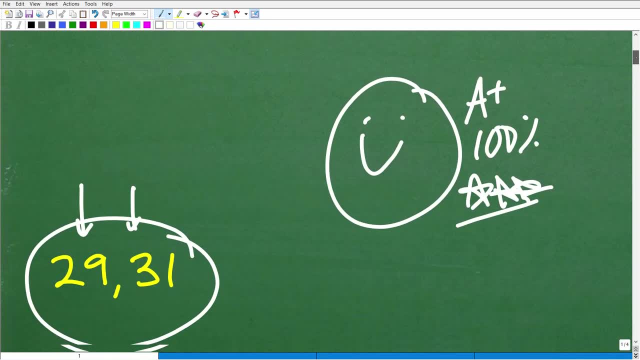 what is a radical? What is a rational number? What is a rational number? What is a rational number? What is an exponent? You know all these different terms you need to kind of remember. you just can't look at math in terms of its patterns and be like, well, that's good enough, I know a lot of. 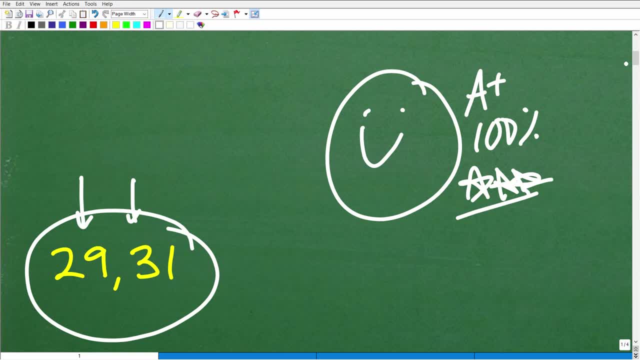 people are like: well, it's one of these things you know, like a polynomial, You might not, you know, remember the actual term to describe something, but you should try to strengthen your math vocabulary. It is very important, But let's go ahead and get into the problem. 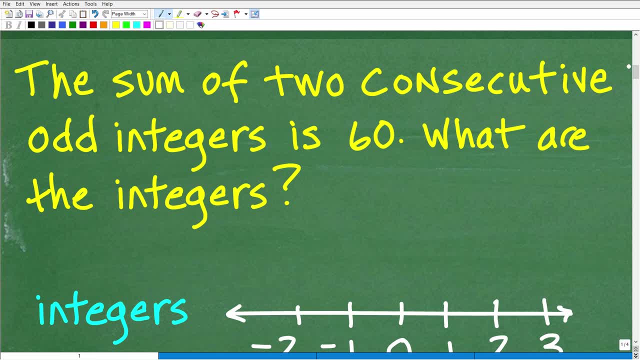 So again we have an algebra word problem Now, in general, okay, when you're solving any word problem in mathematics, you want to read the problem at least three times. I'm going to quickly go through what I feel is like a good kind of set. 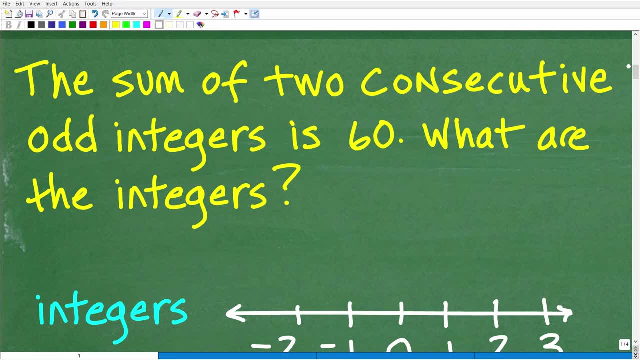 of guidelines here And if you need additional help with word problems or if you want to practice more algebra word problems or just, you know, learn the algebra that you need to solve these word problems. I have additional word problems on my YouTube channel And if you 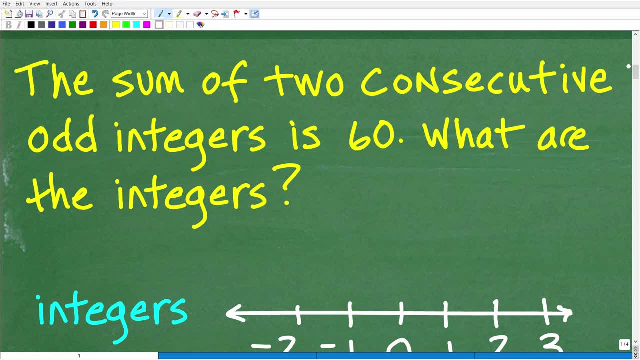 really want to kind of get into all this stuff. check out my YouTube channel And if you want to find math courses, you'll find the links to each of those in the description below as well. So again, you can have more advanced word problems if you're taking pre-calculus versus, you know. 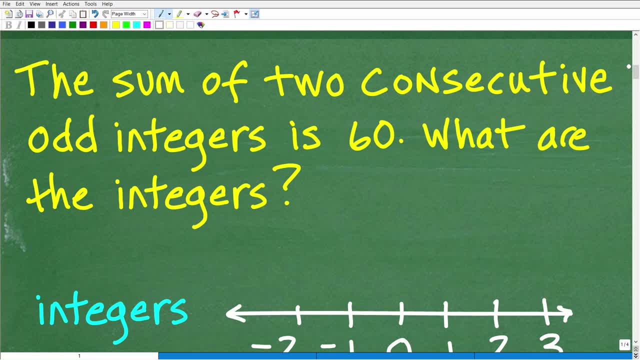 something more basic like this. You'll probably find this particular type of problem like maybe like in a pre-algebra or algebra- one course Okay, but what you want to do is read the problem at least two or three, at least three times, not two or three times, at least three times to make sure. 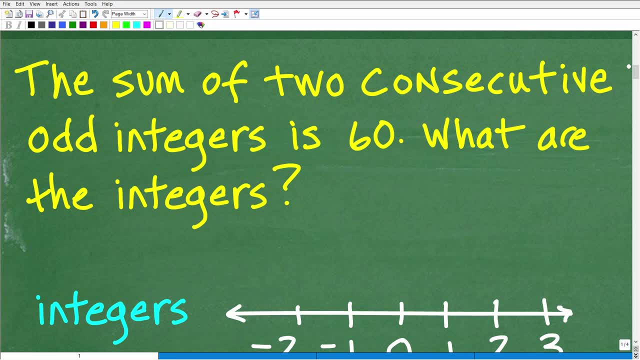 you fully understand what's going on. So that's step one. Step two is: you want to kind of model this situation. Okay, you can kind of graphically do that, but any kind of creative way, so you can kind of visually see what's going on or try to you. 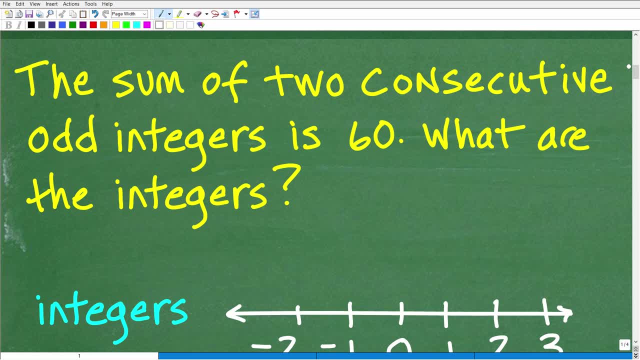 know kind of see patterns that you need to understand in order to figure out the problem. The third thing is you want to establish a variable. The fourth thing is you want to create an equation. okay, to solve for that particular variable. The variable is going to represent. 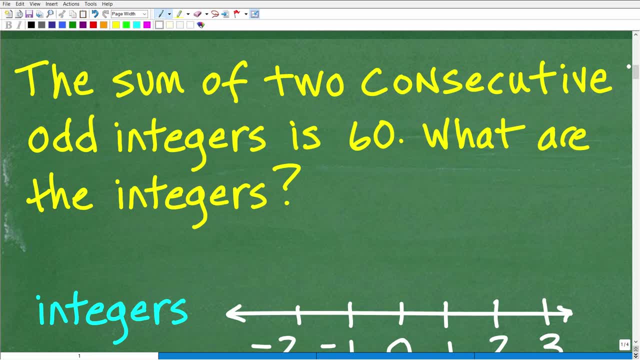 you know the unknown values that you're trying to solve for Okay, and then you're going to solve the particular equation that you set up and then you're going to answer the question. So I didn't list these things out. I'm just kind of telling you these guidelines here. but anyways, let's go. 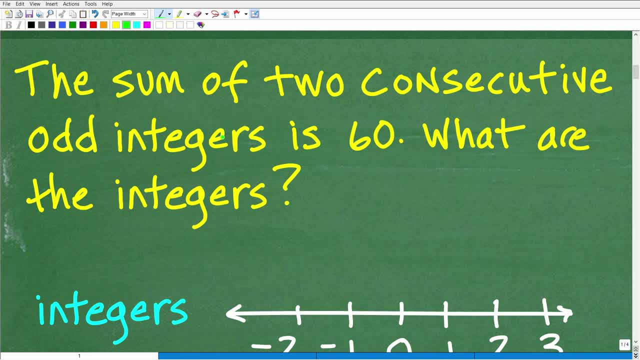 ahead and get into the problem, and before we go any further, let's make sure you understand what an integer is and then what this word consecutive means, because if you don't understand these terms, you're not going to be able to do this problem. So integers, okay, in mathematics, remember these. 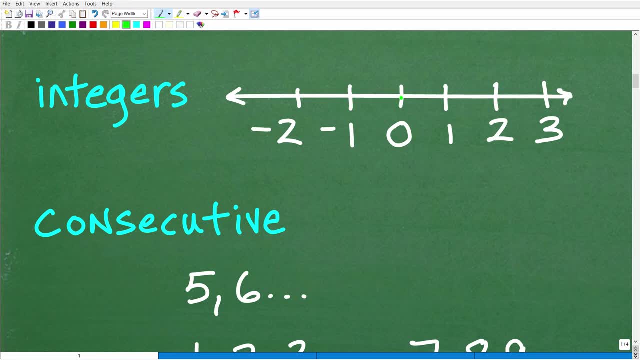 and it's these numbers right here. okay, So we can start with zero. So we got one, two, three. Now, typically, if it was just one, two, three, you would just describe these numbers as you know. 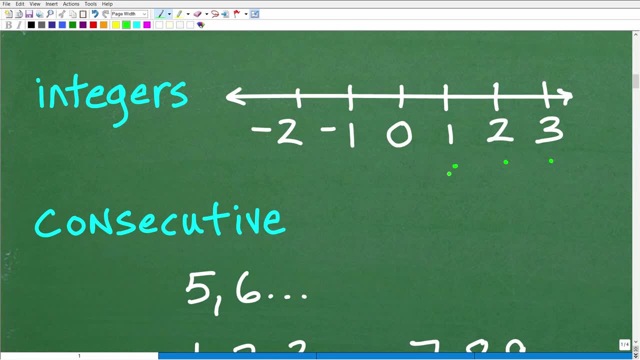 these would be what we call the counting numbers, okay, or natural numbers. Then we throw in zero, then we have the whole numbers and then if you take the positive and negative, the whole numbers, you have the integers. but you can just kind of remember: you got one, two, three, zero. 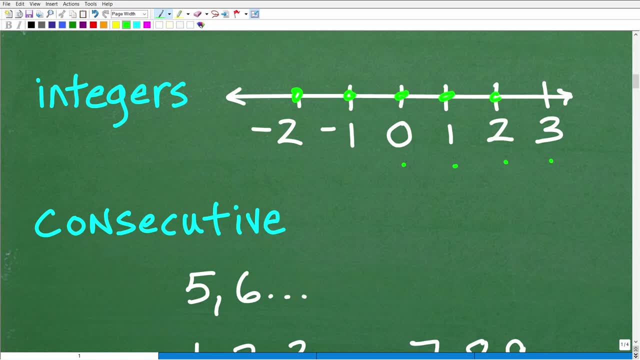 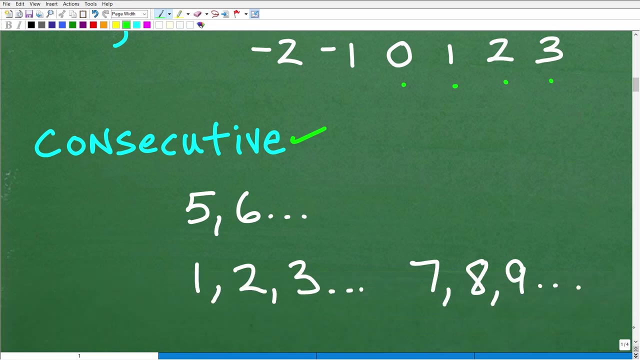 negative one, negative two. These numbers like this are integers. okay, and of course they continue on in both directions. Okay, so that's what an integer is. and consecutive? well, the word consecutive in mathematics or anything is just. you basically have one thing right after a number. 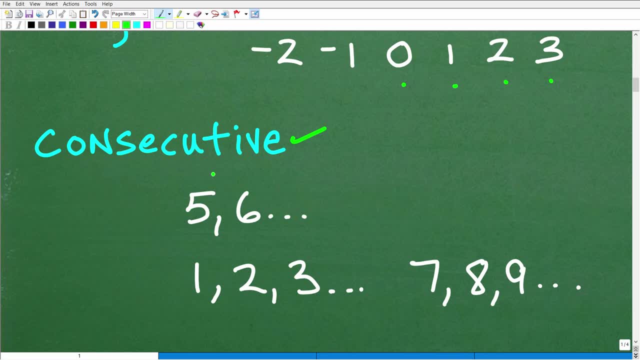 that comes right after a previous number, right? So you have a number and then the next number. I guess that's the best way to say it. I'm not going to give you like a formal definition, Easier to see it. So five and six are consecutive numbers, right? So you got five and then the next. 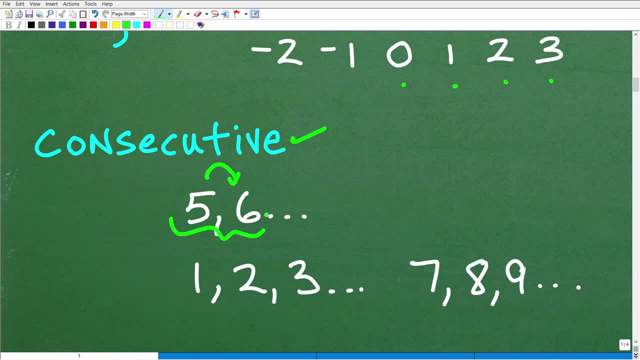 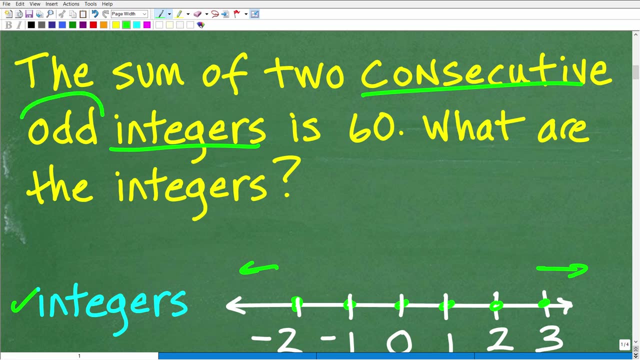 number is six, So you would describe these numbers as consecutive. Now this problem is a little bit different, because we're not talking about consecutive numbers. We're talking about consecutive odd integers. So we have to kind of think about this for a second. So let's take a. 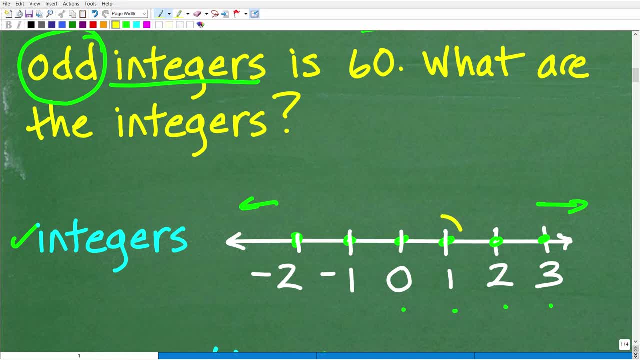 look at some examples of consecutive odd integers. Like if we have one, okay, one is an integer. I have an integer and one is odd. So the next number, the next integer, is two. but that's even okay, So that's not going to be good. So here, three. the next number comes after. that is odd. 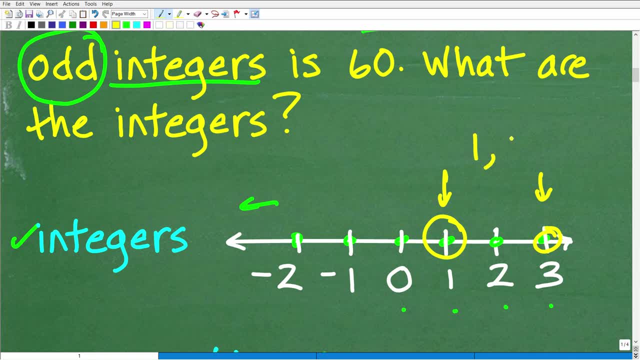 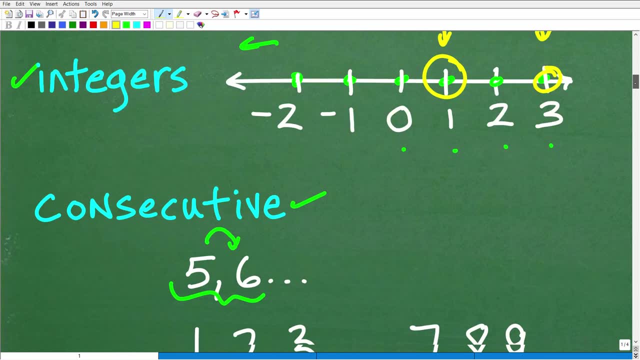 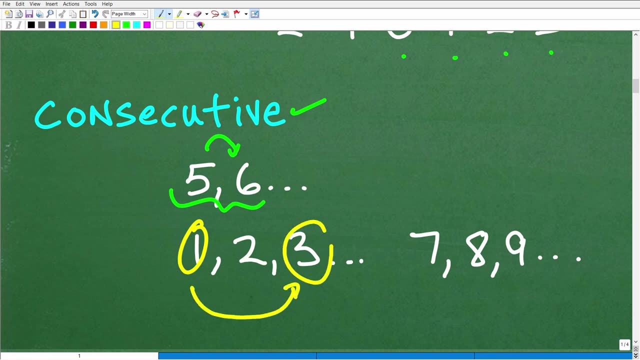 and it's an integer, So consecutive odd integers would be like one and three, okay, So you got to really make sure you understand that, all right, Okay, So over here you can see that if I have consecutive odd integers, the next consecutive odd integer would be three. okay, You can see this. 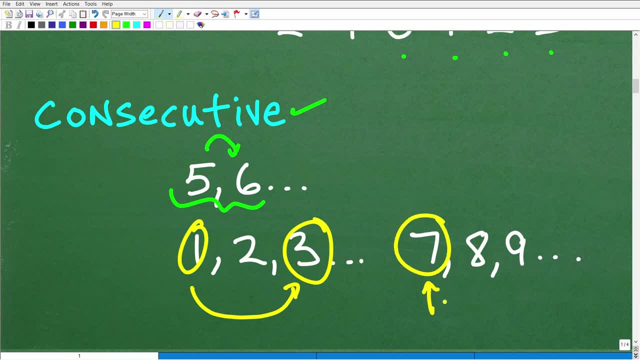 pattern here. So seven is an integer, It's odd. So the next number is eight, It's even. So the next number after that is odd. So like seven and nine would be consecutive odd integers. Now if 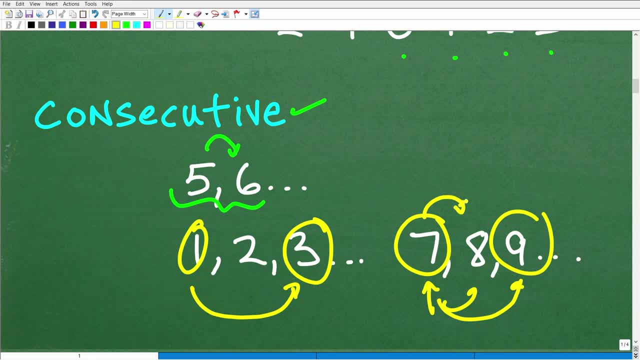 you notice, here they're separated like consecutive numbers. All you have to do is add one to get the consecutive integers. to get to the next number, right, But to get to the next consecutive odd integer- excuse me, to get to the next number, you have to add one to get to the next number. So 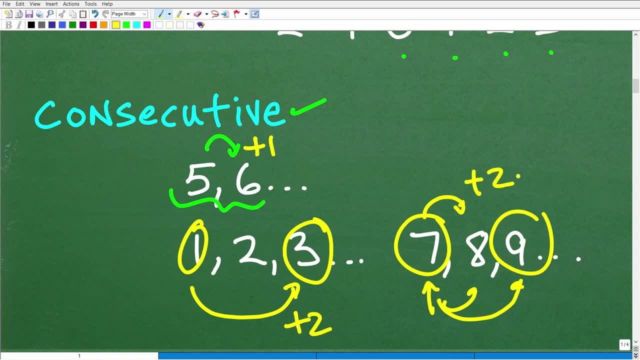 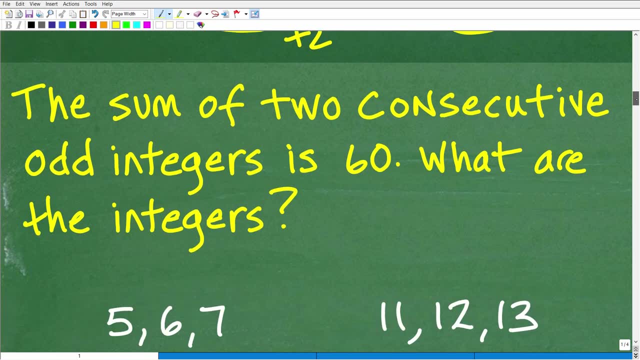 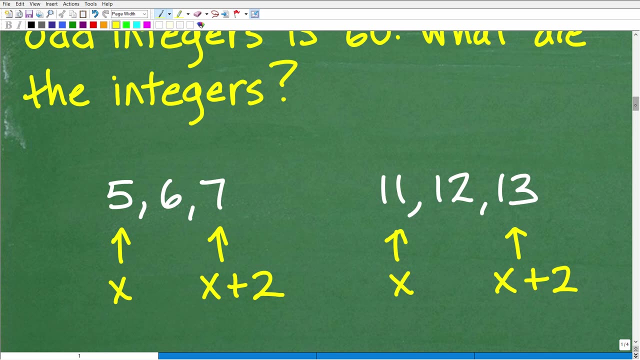 you have to add two, And so it's important that you kind of model- you know patterns here so you can understand what you need to do. And so what we're going to do now is establish a variable right So we kind of hopefully understand the pattern. here We're looking for two consecutive 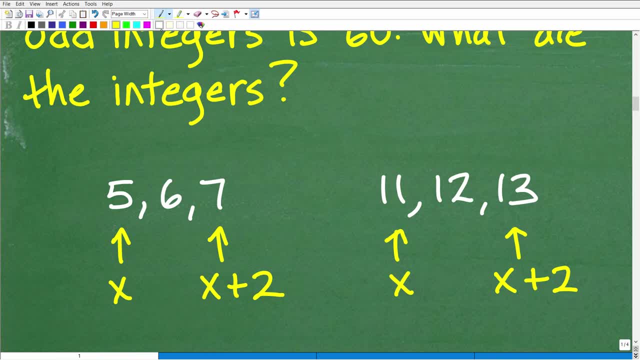 odd integers. So if we let our first integer be like x, right, X represents an unknown value. whatever that is, If x is our first odd integer, then x plus two will be our next integer right, Our consecutive odd integer. So if x is our first odd integer, x plus two is the consecutive odd integer right. 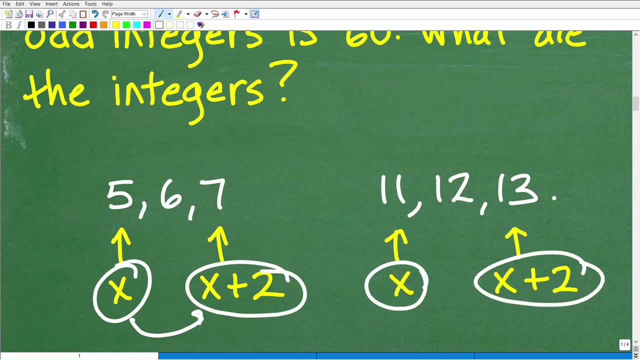 And you can see this pattern play out with any set of you know integers right, Like 11,, 12, 13.. These are integers Odd, odd, just you know, just whatever your integer is, x. 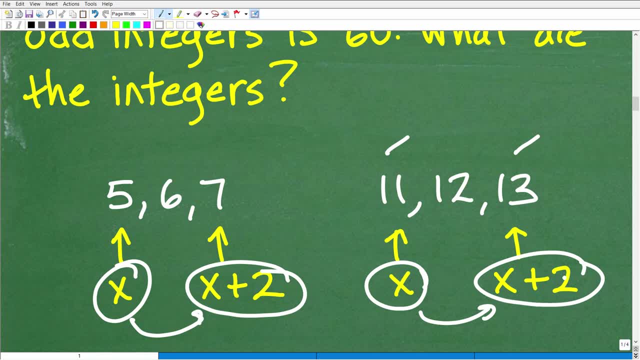 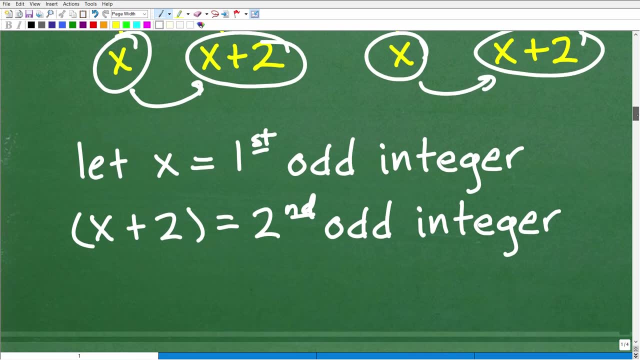 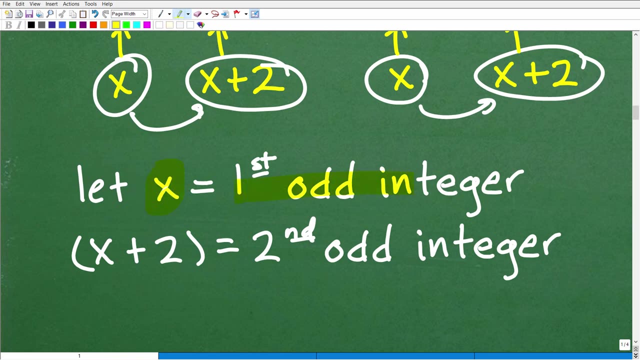 add two to it and you get your next odd integer right, Consecutive odd integer- Okay. So now that you understand the pattern, let's go ahead and formalize this and kind of define variables. So we're going to go ahead and let x, okay, be equal to the first odd integer, So x plus two will be. 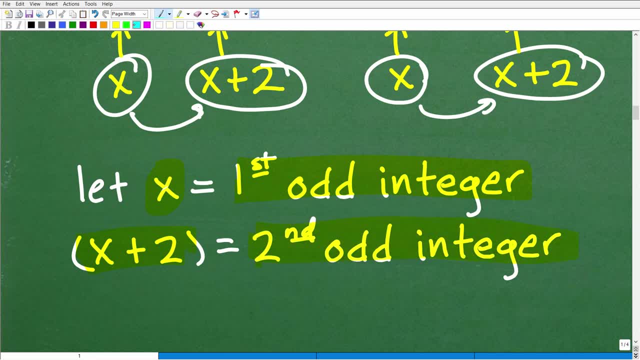 our second odd integer. Now a lot of you might be saying: well boy, you're really dragging this out. Mr YouTube, Math Man, I get what you, I get what you know what I need to do here. But 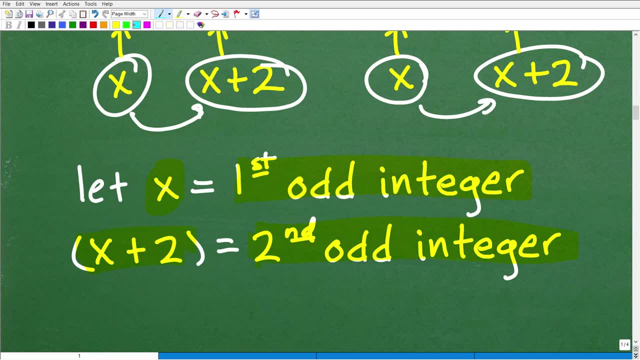 you don't need to write all this stuff out. Listen, this is the way you know you get better at word prompts. This is a basic word prompt and you know you need to kind of tell the story of how you're solving it so your teacher or anyone else can understand what's going on. So if you 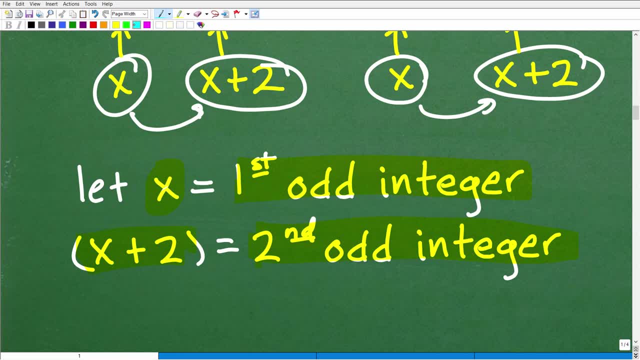 can't you know kind of structure your solutions properly in easy word prompts like this? you're going to have a tough time with more advanced word prompts. So label things, just follow the kind of the guidance I'm giving you. So establish what these variables stand. 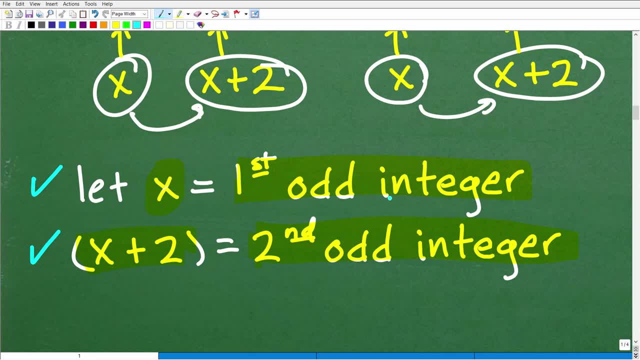 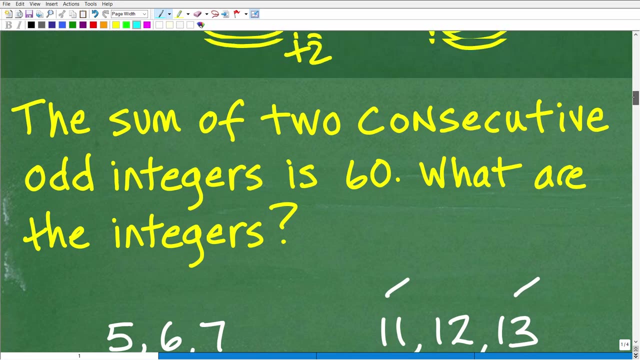 for. So let x equal. just write this down: the first odd integer, So x plus two will be the second odd integer. Remember, we're looking for two odd integers, So we'll have our first number and our second number. Okay, So now we need to kind of go back up to this part of the problem. 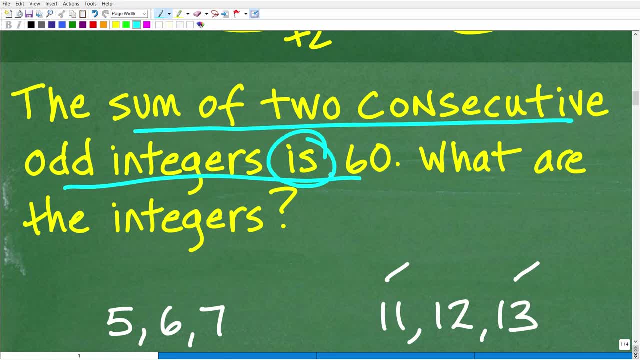 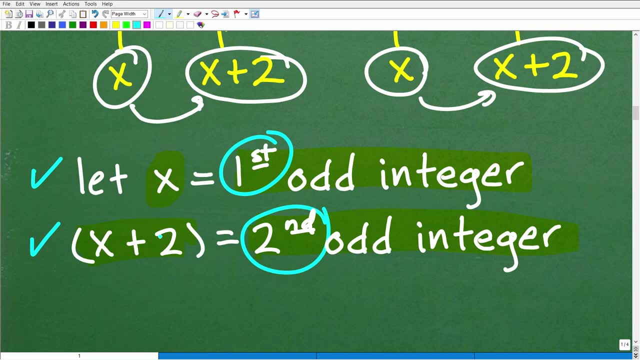 The sum of two consecutive odd integers is or is equal to 60.. All right, So now we're going to go ahead and build an equation. So we have these variables, but in order to do that, we're going to have to solve for these unknown values. We need to set up an equation, So here is our. 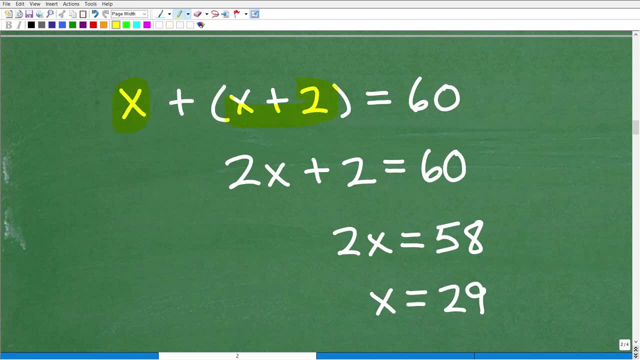 equation. So here is our first odd integer and this is our second odd integer. right here, right. So we have x and x plus two. The sum of these two odd integers is 60.. All right, Okay, So now. 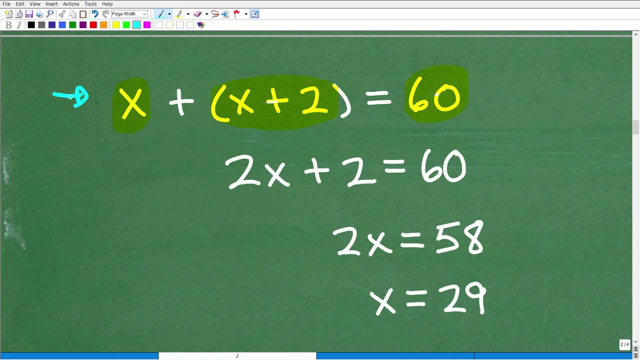 that you're satisfied you got the correct equation. you model this situation. Now. we're just kind of off to the races to solve this nice basic linear equation. so I have: x plus x plus two is equal to 60. So x plus x is 2x plus two is equal to 60. Now 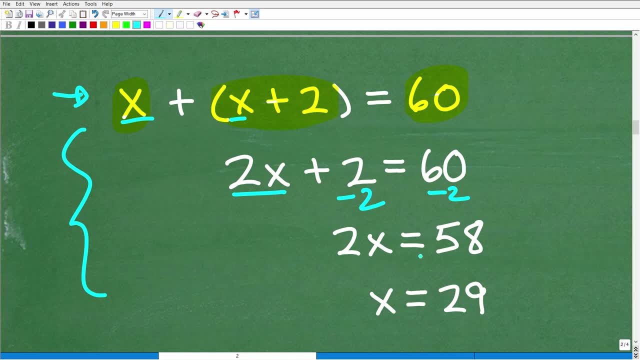 I'm going to subtract two from both sides of the equation and you're going to get 2x is equal to 58. So to solve for x, all I need to do is divide the equation- both sides of the equation- by two. 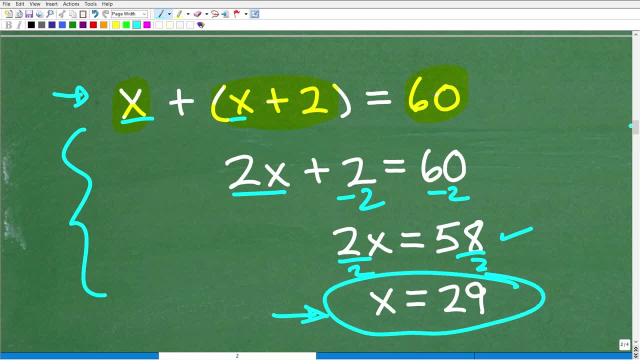 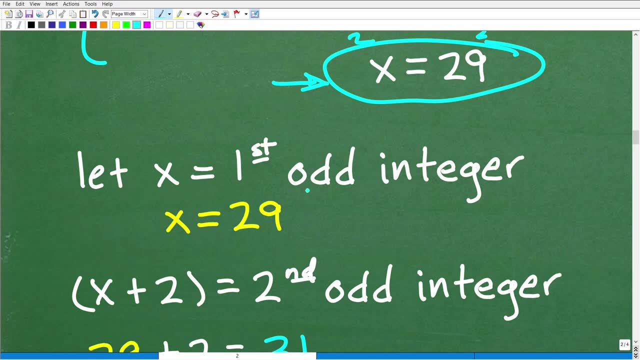 excuse me, and you get: x is equal to 29.. Okay, So what does that mean, though? Well, let's go back to you know when we established our variables, right, The first odd integer, So our first odd integer, is 29,, and we just kind of deduce that. the plus two: 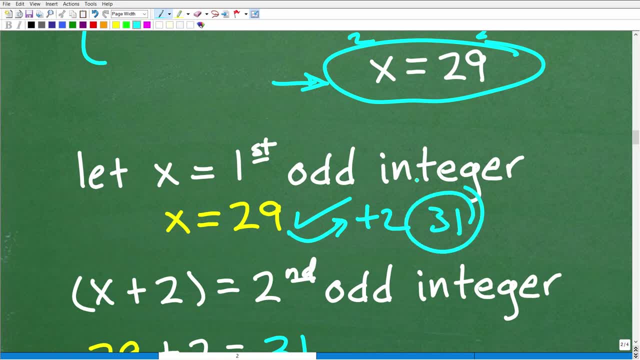 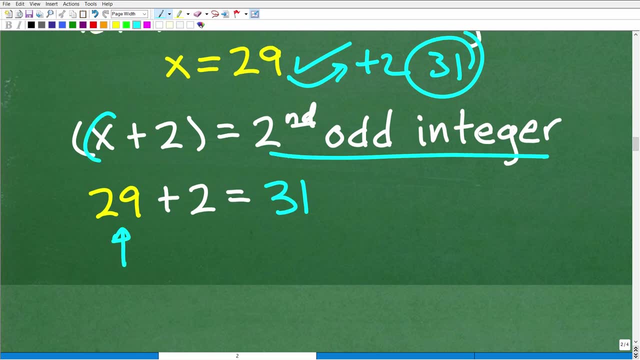 okay, when we add two to this one, we're going to get to our second one, which is 31.. And of course we kind of formalize that right here. So x plus two is our second odd integer. Our first integer is 29.. So it's 29 plus two, That is 31.. Okay, So again you know pretty. 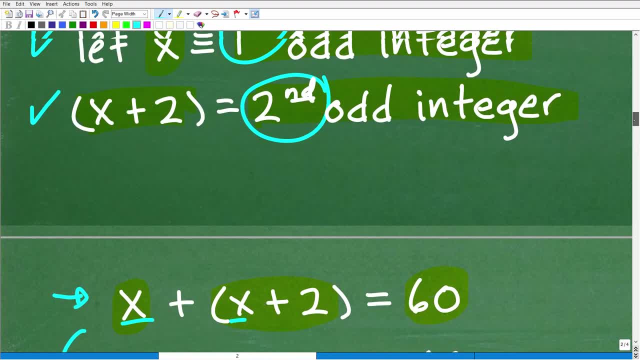 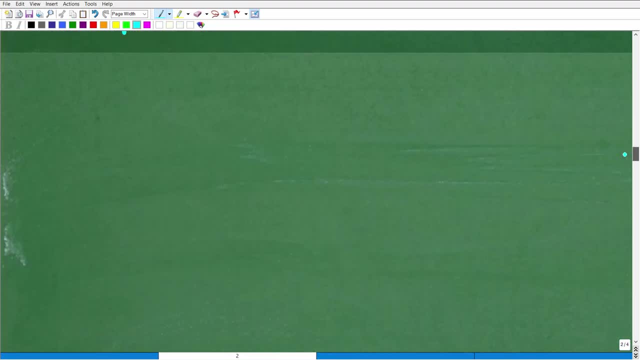 hopefully not too difficult of a problem to understand, Even if you didn't get it right, you know. if you understand it, you know that's excellent. And I want to make another kind of point here as well. Now, if you're watching this video, well obviously you're. 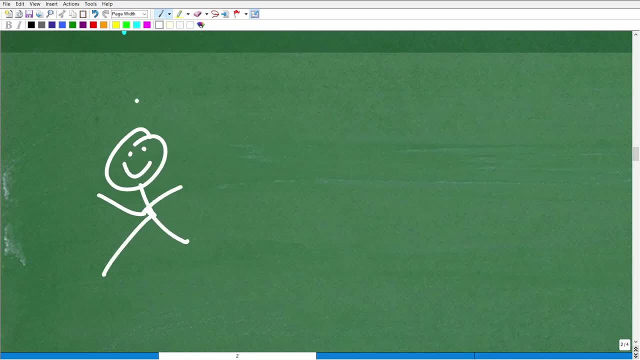 watching this video. So here you are. Hopefully you got a smiley face on and your brain is working and you're like, wow, that was pretty cool And you're watching. you're watching me do the work, right? You're watching me work and you're watching me solve the problem and you're.